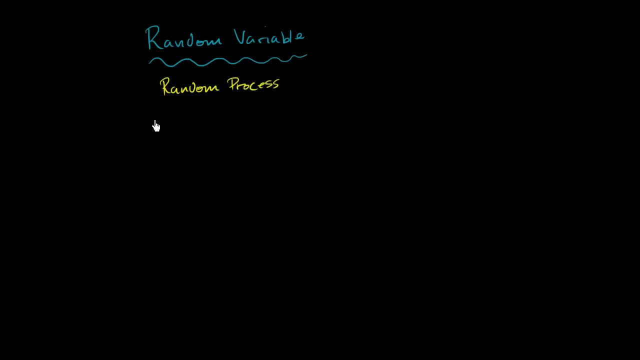 so random process. you are really just mapping outcomes of that to numbers. You're quantifying the outcomes. So what's an example of a random variable? Well, let's define one right over here. So I'm going to define random variable: capital X. 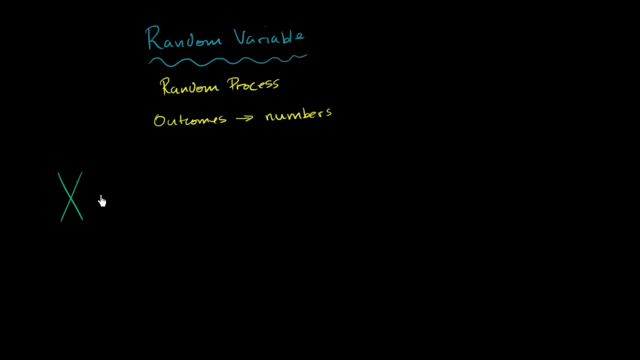 And they tend to be denoted by capital letters. So the random variable, capital X, I will define it as is going to be equal to 1 if my fair die rolls heads, And it's going to be equal to 0 if tails. 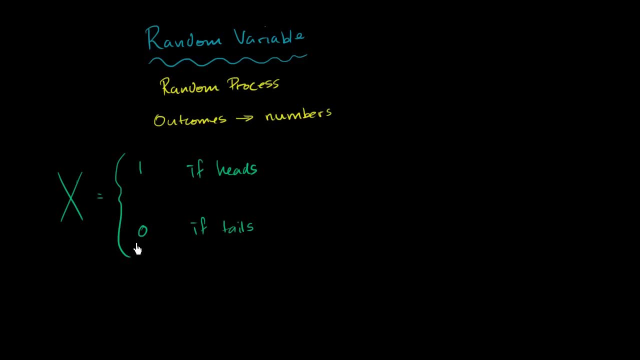 I could have defined this any way I wanted to. This is actually a fairly typical way of defining a random variable, especially for a coin flip. But I could have defined this as 100, and I could have defined this as 703.. And this would still be a legitimate random variable. 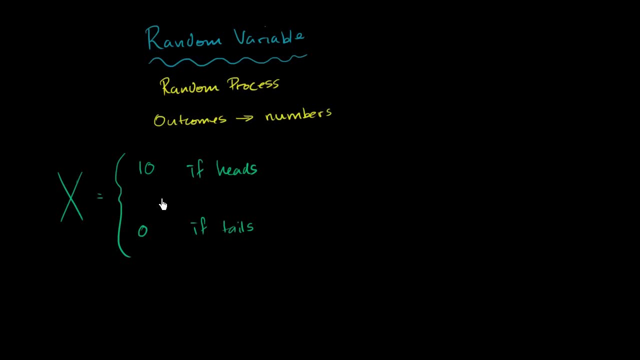 It might not be as pure a way of thinking about it as defining 1 as heads and 0 as tails, but that would have been a random variable. Notice we have taken this random process flipping a coin and we've mapped the outcomes of that random process. 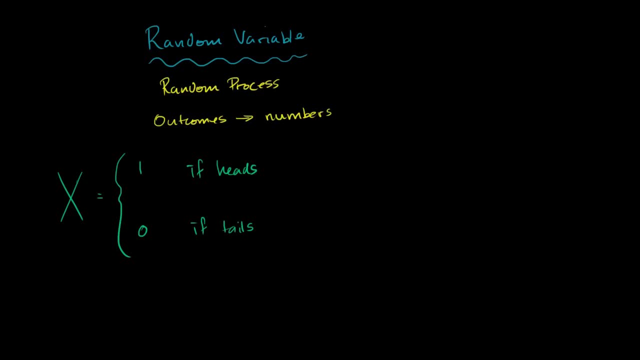 And we've quantified them: 1 if heads, 0 if tails. We can define another random variable, capital Y. So capital Y is equal to, let's say, the sum of rolls of, let's say, 7 dice. 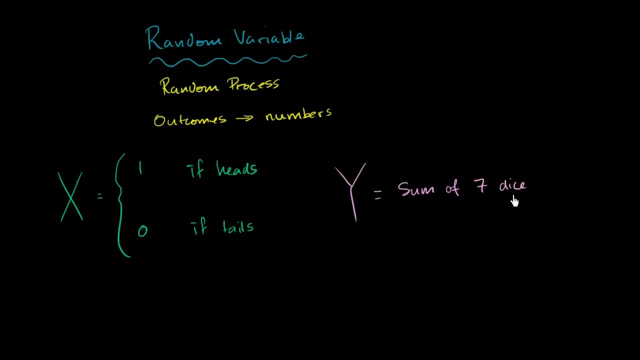 And when we talk about the sum, we're talking about the sum of the 7.. Let me write this: The sum of the upward face after rolling 7 dice. Once again, we are quantifying an outcome for a random process. 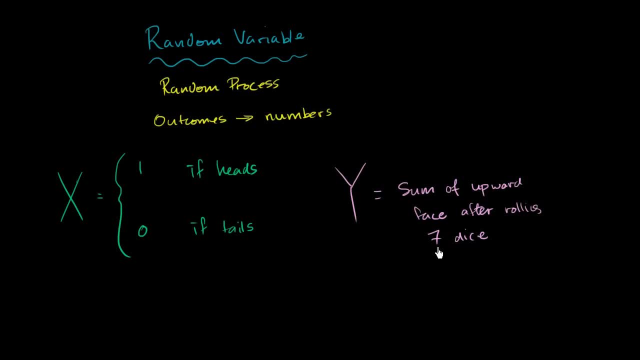 The random process is rolling these 7 dice and seeing what sides show up on top, And then we are taking those and we're taking the sum and we are defining a random variable in that way. So the natural question you might ask is: why are we doing this? 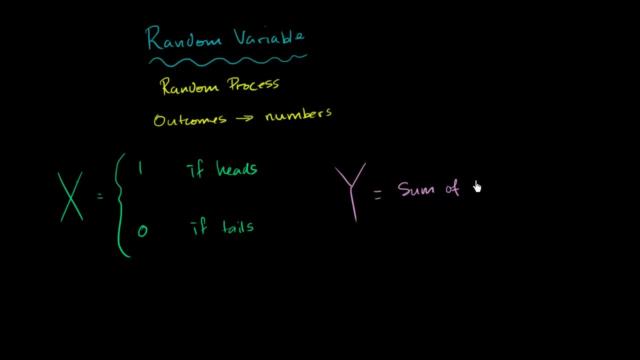 the sum of rolls of, let's say, 7 dice. And when we talk about the sum, we're talking about the sum of the 7.. Let me write this: The sum of the upward face after rolling. The sum of the upward face after rolling, 7 dice. 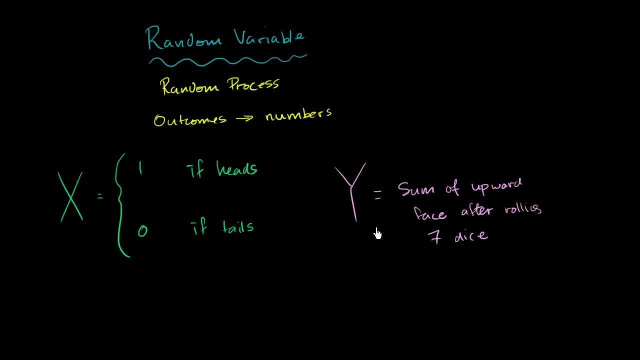 Once again we are quantifying an outcome for a random process. The random process is rolling these 7 dice and seeing what sides show up on top, And then we are taking those and we're taking the sum and we are defining a random variable in that way. 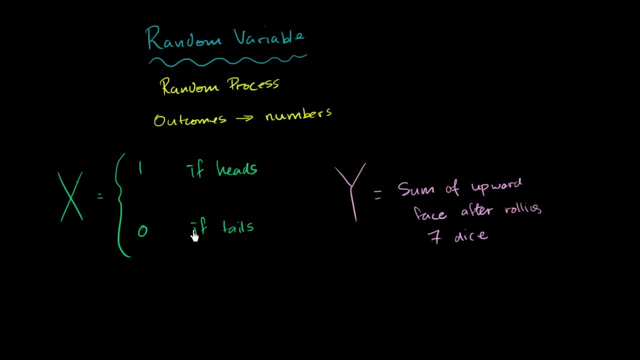 So the natural question you might ask is: why are we doing this? What's so useful about defining random variables like this? It will become clear, It will become more apparent as we get a little bit deeper in probability, But the simple way of thinking about it is: 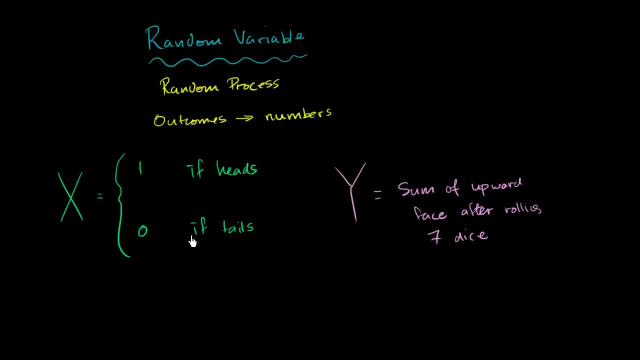 as soon as you quantify outcomes, you can start to do a little bit more math on the outcomes And you can start to use a little bit more of mathematical notation on the outcome. So, for example, if you cared about the probability that the sum of the upward faces after rolling 7 dice, 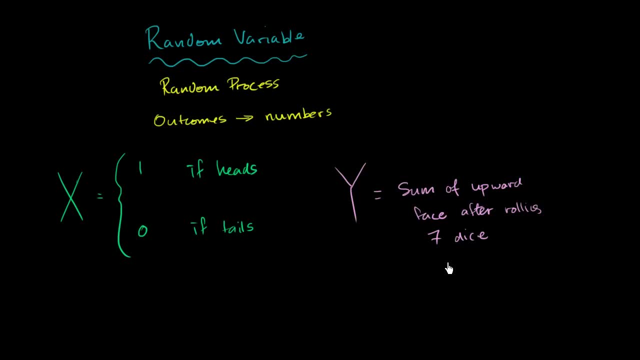 if you cared about the probability that that sum is less than or equal to 30, the old way that you would have to have written it is the probability that the sum of, and you would have to write all of what I just wrote here. 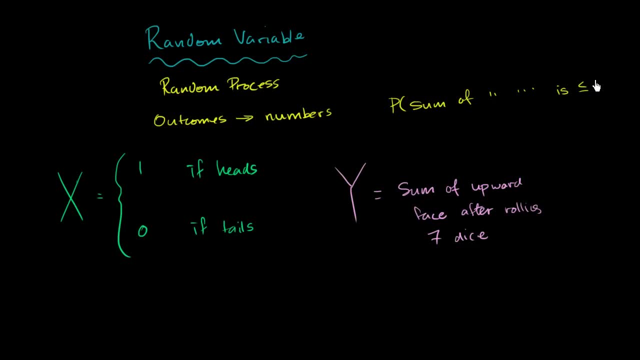 is less than or equal to 30. You would have had to write that big thing And if you wanted to write, and then you would try to figure it out somehow if you had some information. But now we can just write the probability that capital Y is less than or equal to 30.. 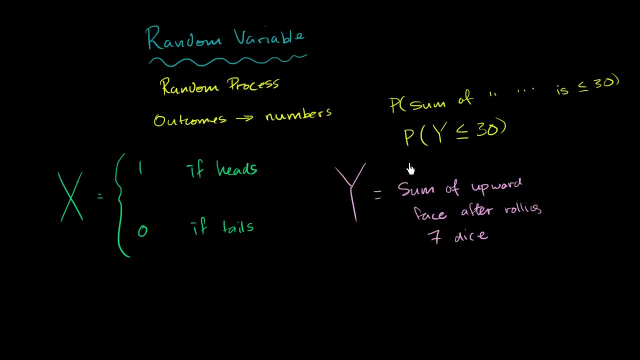 It's a little bit cleaner notation And if someone else cares about the probability that the sum of the upward face after rolling 7 dice, if they say, hey, what's the probability that that's even, instead of having to write all of that over. 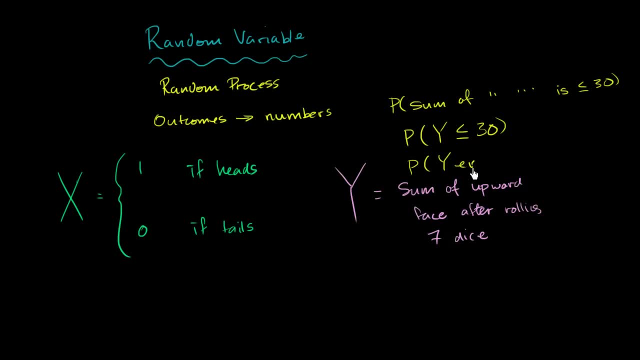 they can say: well, what's the probability that Y is even Now? the one thing that I do want to emphasize is how these are different than traditional variables. Traditional variables that you see in your algebra class, like x plus 5 is equal to 6, usually denoted. 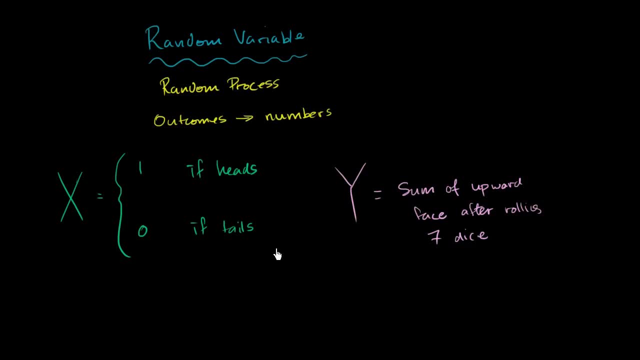 What's so useful about defining random variables like this. It will become more apparent as we get a little bit deeper in probability, But the simple way of thinking about it is: as soon as you quantify outcomes, you can start to do a little bit more math on the outcomes. 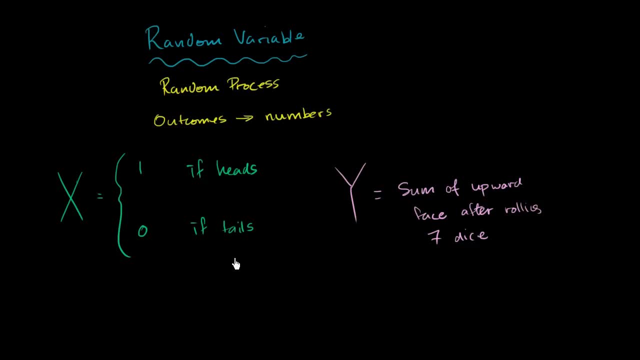 And you can start to use a little bit more of mathematical notation on the outcome. So, for example, if you cared about the probability that the sum of the upward faces after rolling 7 dice, if you cared about the probability that that sum is less than or equal to 30, the old way. 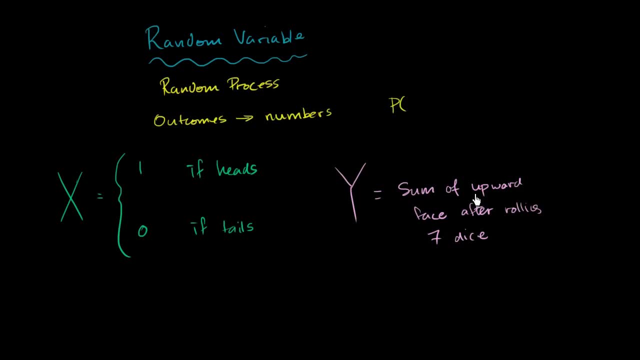 that you would have to. You would have written it as the probability that the sum of and you would have to write all of what I just wrote here is less than or equal to 30. You would have had to write that big thing. 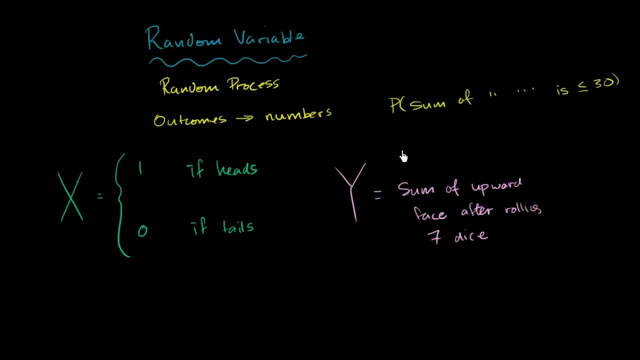 And if you wanted to write, and then you would try to figure it out somehow if you had some information. But now we can just write the probability that capital Y is less than or equal to 30. It's a little bit cleaner notation. 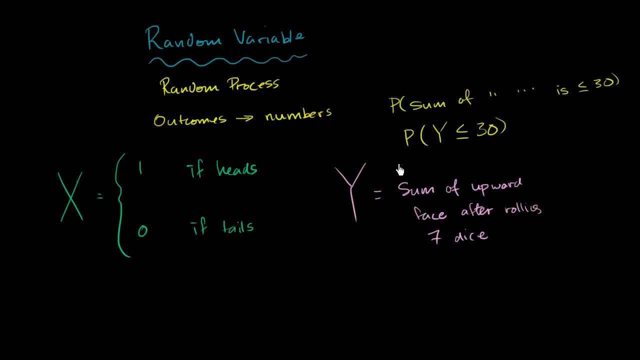 And if someone else cares about the probability that the sum of the upward face after rolling 7 dice. if they say, hey, what's the probability that that's even, instead of having to write all of that over, they can say, well, what's the probability that Y is even? 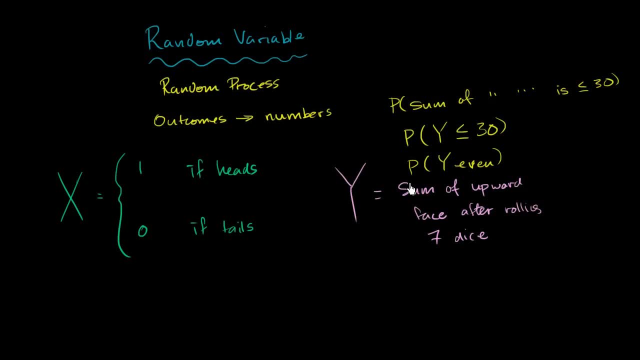 Now the one thing that I do want to emphasize is how these are different than traditional variables. Traditional variables that you see in your algebra class, like x plus 5 is equal to 6, usually denoted by lowercase variables, y is equal to x plus 7.. 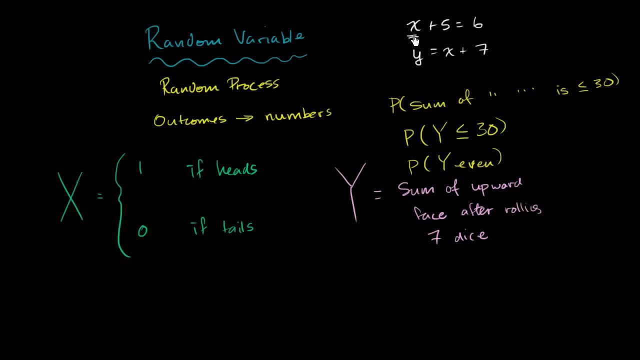 These variables you can essentially assign values. You either can solve for them, So in this case x is an unknown. You can subtract 5 from both sides and solve for x. Say that x is going to be equal to 1.. 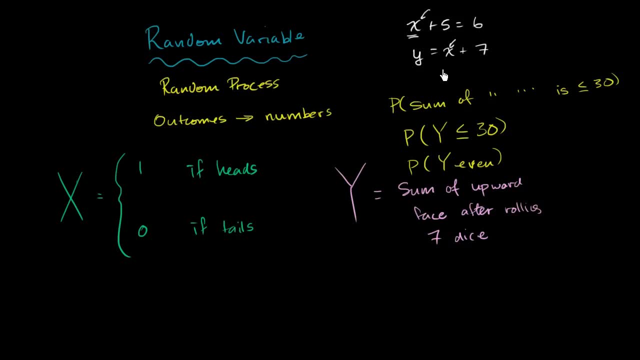 In this case, you could say: well, x is going to vary. We can assign a value to x and see how y varies as a function of x. You can either assign variable, you can assign values to them, or you can solve for them. 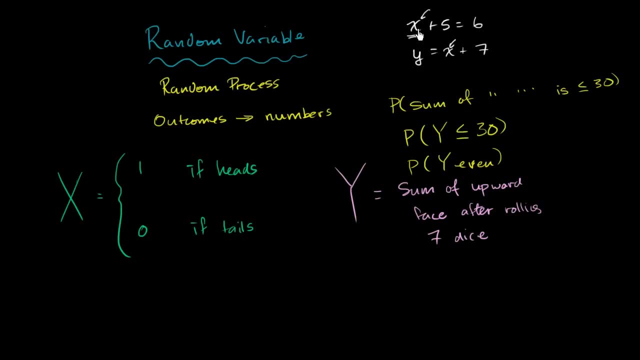 You could say, hey, x is going to be 1 in this case. That's not going to be the case with a random variable. A random variable can take on many, many, many, many, many different values with different probabilities.